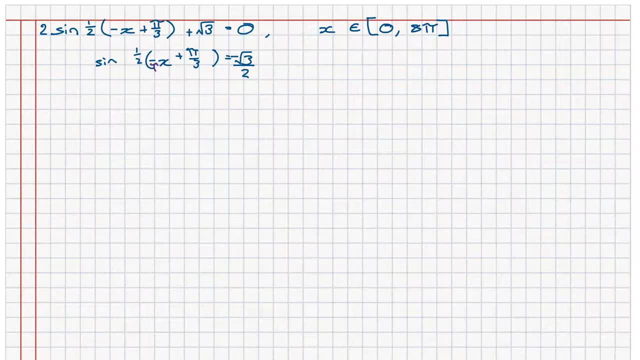 there's a negative in here. If you recall back to the trig identity of negative sine x is equal to sine negative x. what we're going to do is we're going to use this here on the left hand side, and then we're going to divide the right end by 2 and then the left end by 5.. 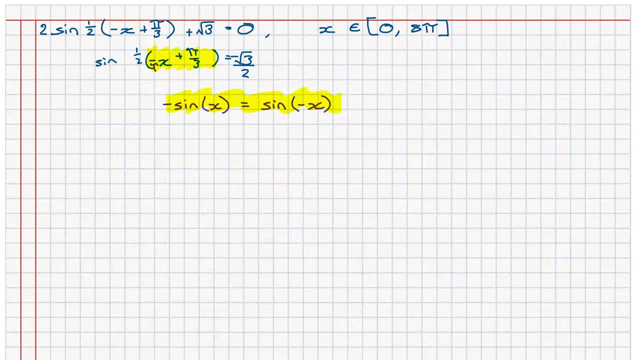 this here to make our equation a little bit easier to work with. so we're going to get this on the right hand side, and then on the left hand side we're going to see negative half X minus pi over 3. as such, then I'm going to apply this. 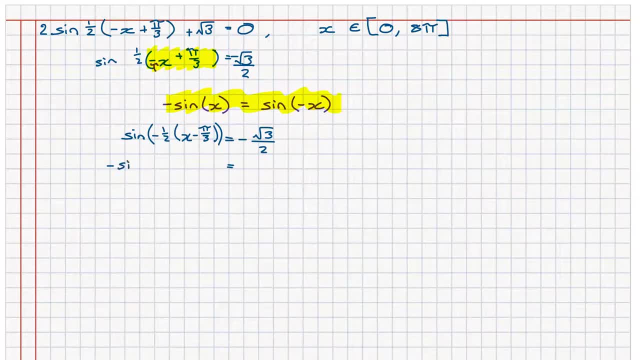 identity above and we'll get negative sign a half X minus pi on 3 and that will be negative root 3 on 2 and then both of these become positive because we can multiply both sides by negative 1. and then the next step is we're going to. 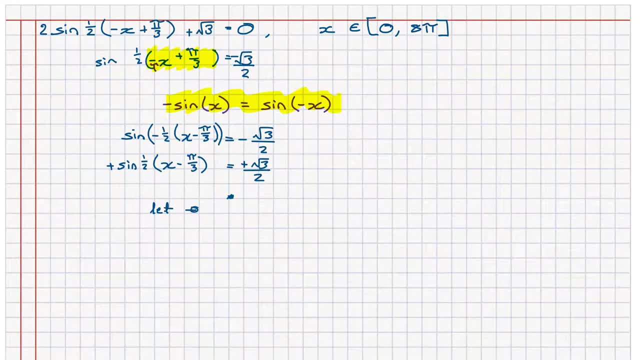 go let theta equal times X minus pi on 3, and then this will remove the translation and the dilation, just for now. so what we're left with is a form that's much easier to work with. so sure, we all feel much comfortable solving this particular problem here now using the unit circle, as always. 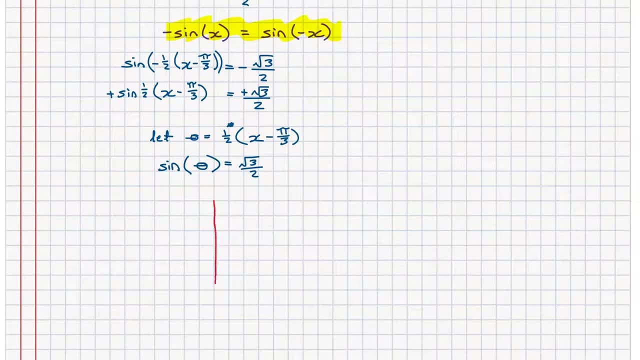 together we're going to get negative. half X minus pi over 3. as such, then we're going to get negative. so sure, we all feel much comfortable solving this particular problem here now using the unit circle. We can use ourgo bloody Testament 2.. So quadrant 1, it's just going to be theta, and then to explain this interior angle here for 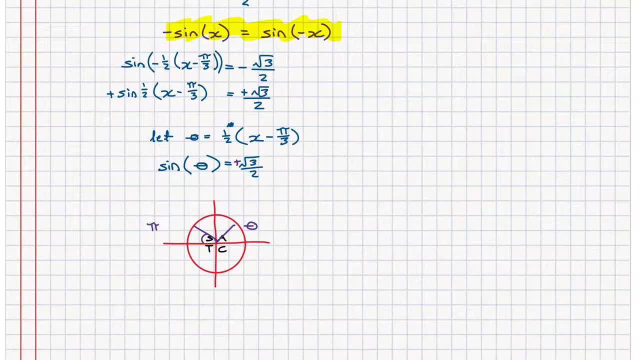 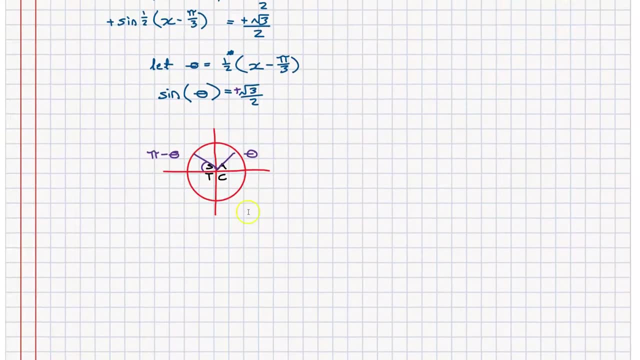 quadrant 2, it's going to be pi minus theta. So the first solution for this particular problem is going to be: theta equals the inverse sine function of root 3 over 2, and we all know from the exact values or simply by memorizing the exact values for at least the. 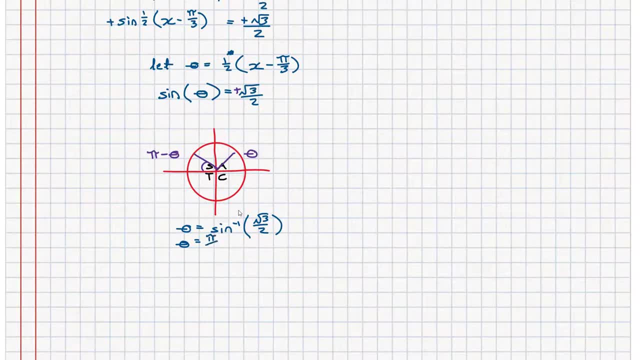 first quadrant. the first solution is going to be pi over 3 radians and then our- well, actually I should mark that as first solution, just so the marker knows that we know what we're doing. then our second one is going to be theta, but rather: pi on 3 equals pi minus theta, and we're after theta as always. so theta is going. 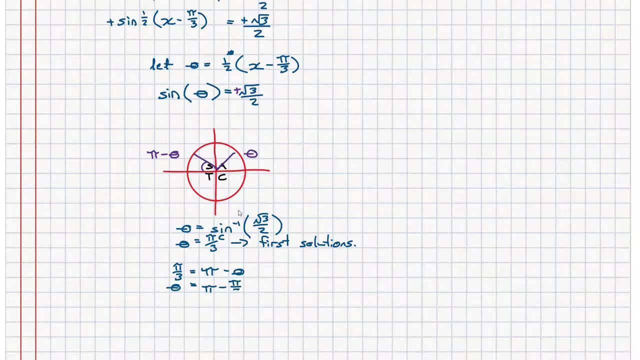 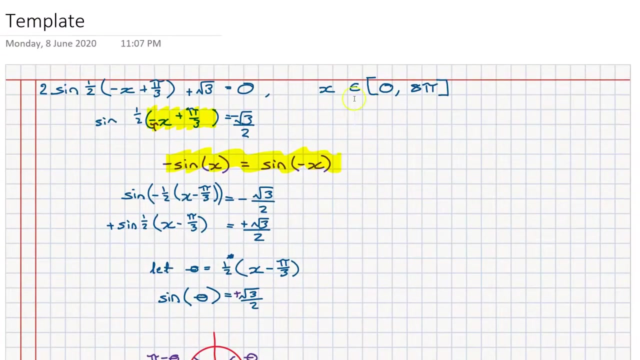 to be pi minus pi on 3, and that will simply equal out to 2 pi over 3 radians. and this will be our second, our second solution now, in the past, when I've done these sort of problems, I've always gone up and I've grabbed. 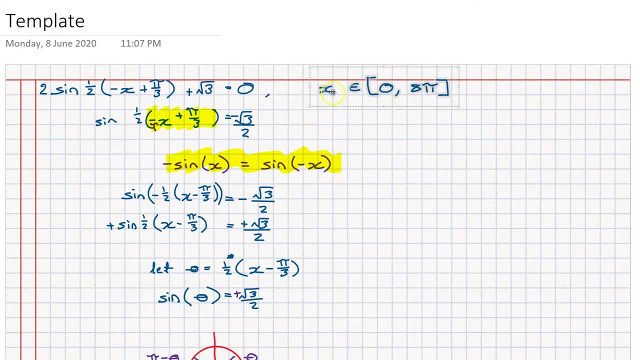 the domain and I've changed it in terms of, so in this case it's x, but down here we're working in terms of theta. so in the past what I'd been doing is I'd been, I'd been changing the domain here to be in terms of theta, but for this particular question I'm not going to do it, and the reason 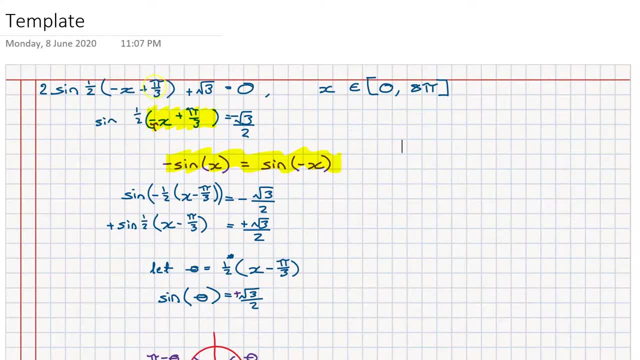 I'm not going to do it for this question is because I'm not going to do it for this question is because we've got this horizontal translation here. so what this horizontal translation will do is it will make it will make us have to do a number of different calculations to change this. 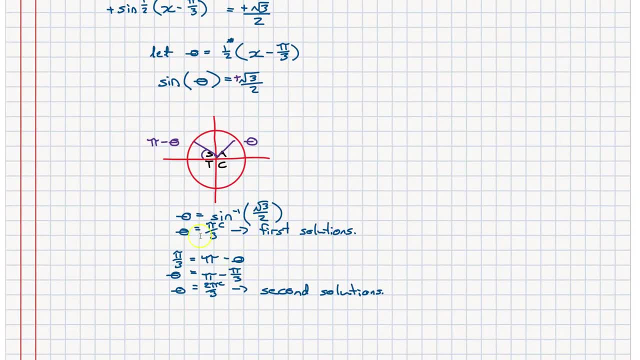 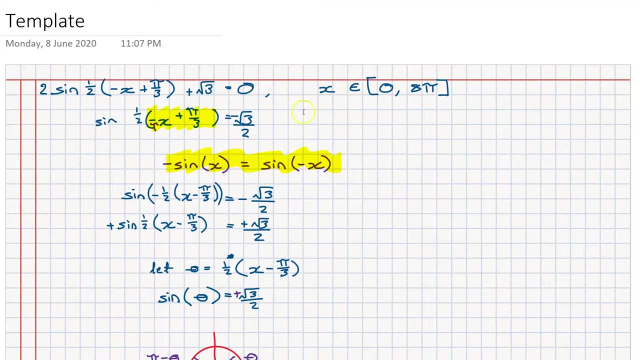 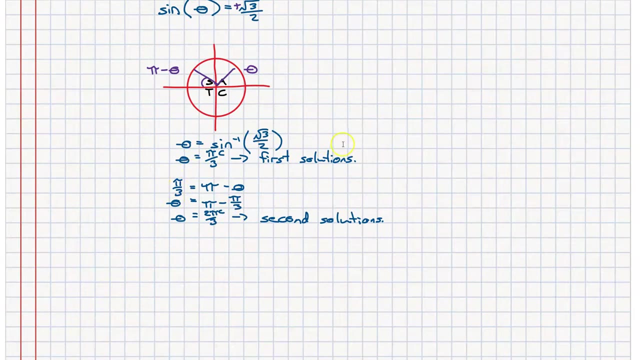 domain around, get all the solutions, verify we're in the correct area or all our solutions are valid, and then to go back. it's actually a bit quicker to sort of ignore the domain for now. calculate all of the solutions in terms of theta, go back and do the same thing over and over and 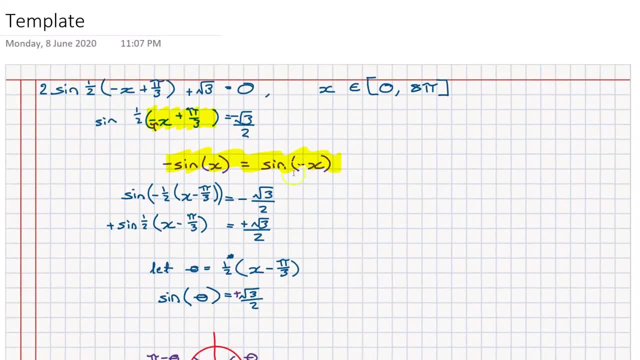 go back to being in terms of x and then verify whether you've got all of your solutions or not once you're back in x. if you don't have them, then you can go back and find more. or if you've exceeded the the constraints of the domain, you can clip them off. but it's purely a time choice here of 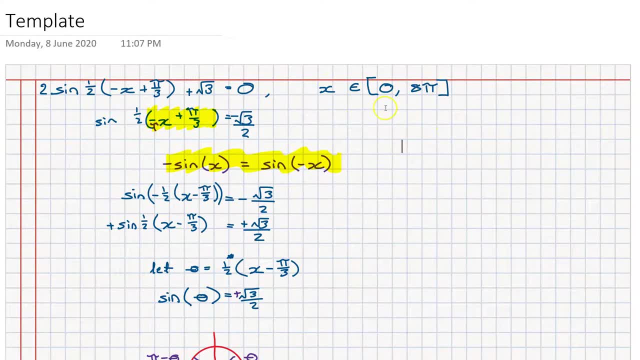 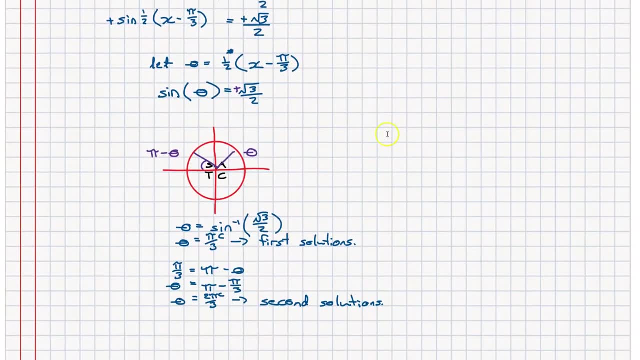 ignoring the domain for now. of course, you can do it with the previous questions as well, but again, the the time factor is not as critical as when you're doing these sort of questions here. so, moving on and ignoring the domain just for now, what we're going to write is: 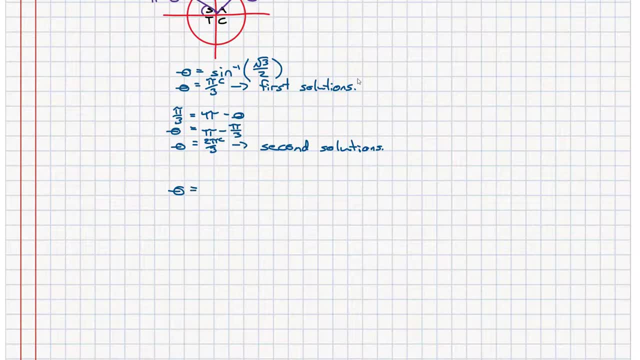 theta equals pi on 3 plus 2k pi. and then the second solution is 2 pi on 3 plus 2k pi, and we have to explain what k is. so we're going to say where, where k is a positive integer between zero and one. now the next question might be: well, how do i know it's between zero and one? 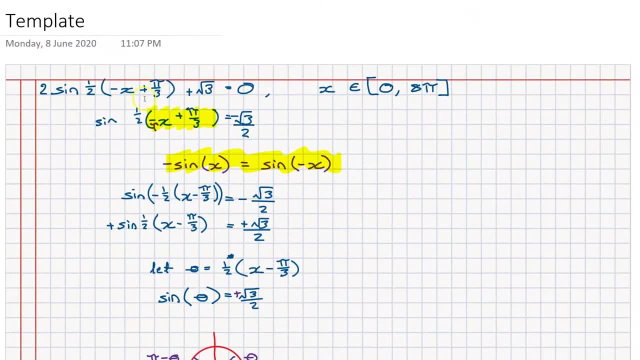 and again. that's simply by looking at the original question posed here and then factored down to, let's say, just before we started working in terms of feed us our highlighter in green. so where is it? this guy, here and here and the original domain here. so, going across, we ask ourselves what's the period going to be for this particular 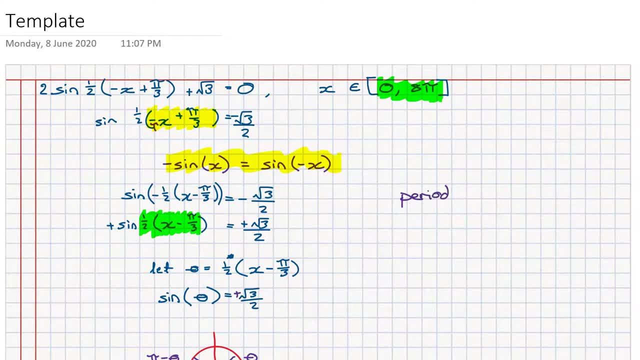 function and the period is going to be 2 pi divided by n, and in this case is a half. so what we're going to get is a period of 4 pi. and then the next question is: well, how many cycles are we expecting? and it's going to be 8 pi minus 0, all over 4 pi, and that's going to be reduced down to 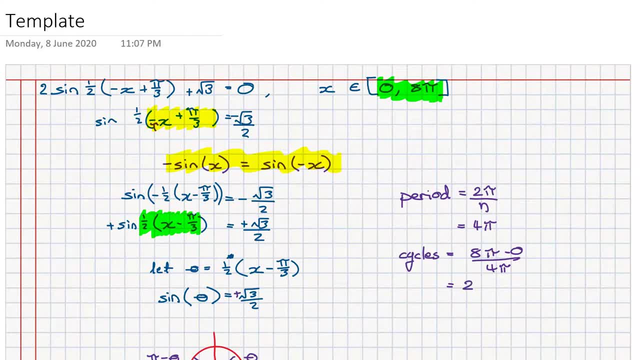 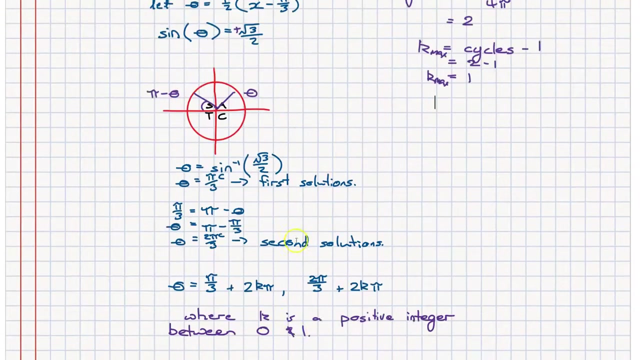 we're going to get 2 cycles and k, and k is equal to the number of cycles minus 1. so 2 minus 1 is simply 1. so whoops, I should say maximum value of k. so that's where our 0 and 1 come from. here again, 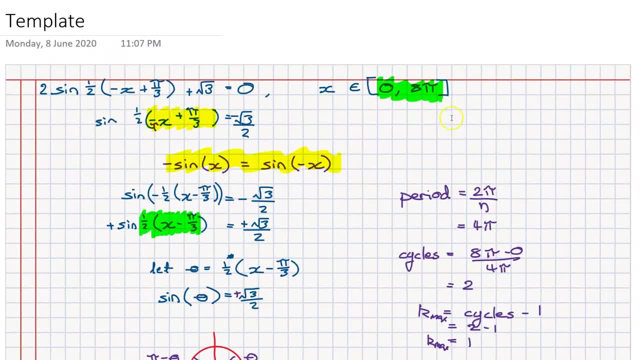 we don't have to explain this bit. it's sort of assumed that you can work it out based on the don't do it again. but it's sort of assumed that you can work it out based on the don't do it again. don't do it again. but it's sort of assumed that you can work it out based on the don't do it again. 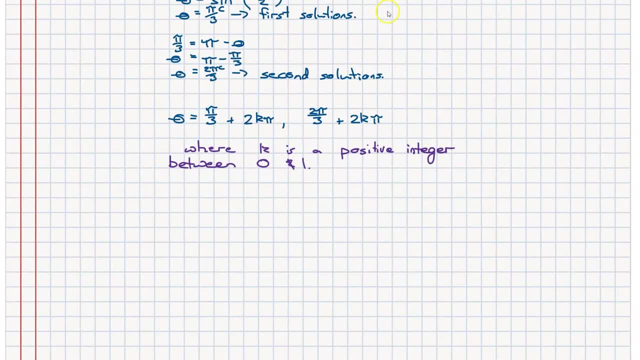 main up here. now, moving onwards, what we can say is: whoops, a thinner pen, rather than going and working out all of these solutions. so, doing this, we're going to get a half. a half X minus pi on 3 is equal to pi on 3, and we're going to get a half x minus pi on 3, and we're going to get a half x. 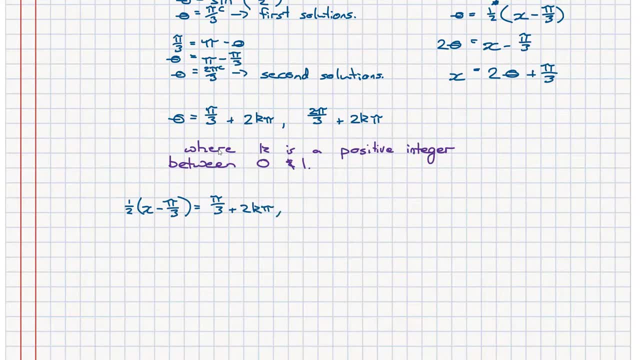 plus 2k pi, and then 2 pi on 3 plus 2k pi, and then we need to have a common denominator here. so we're going to get 3, that's going to be pi on 6k pi, then 3, again 2 pi plus 6k pi, then multiplying both sides by 2 to get rid of the half. 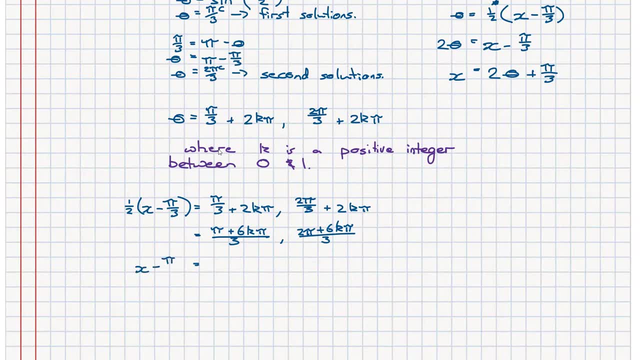 on the left hand side we're going to get x equals pi on 3. then this will become: do it over two lines: 2 pi plus 12k pi and then similarly 4 pi plus 12 K pi. then we have to deal with this phase here. so I'm going to add pi on 3 to both. 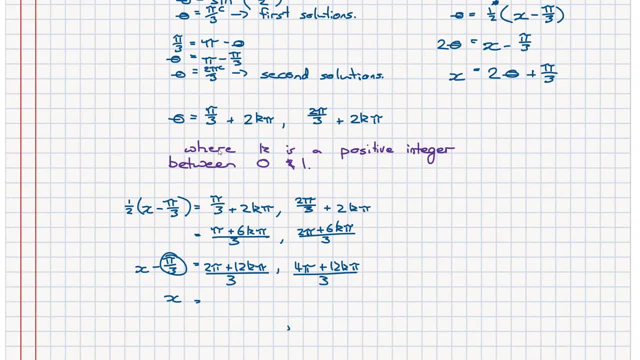 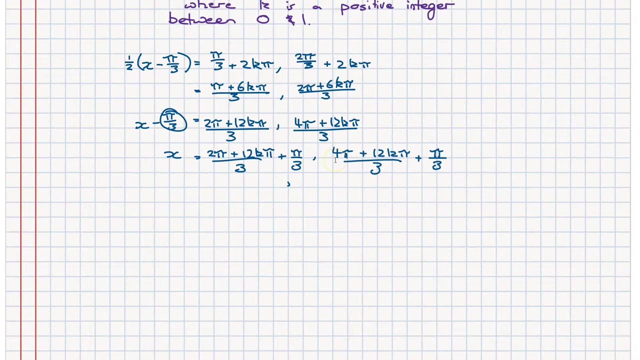 sides of the equation. so what that will evaluate at 2 will be 2 pi- very good, very good- plus 12k pi all over 3 plus pi over 3, and then we're going to have 4 pi plus 12k pi, 3 plus pi over 3, and continuing onwards. this will evaluate to be- luckily these are in- 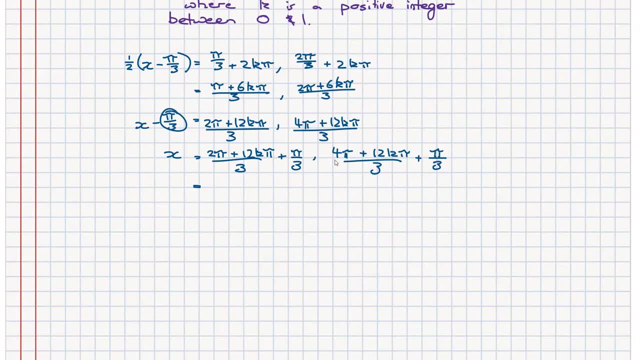 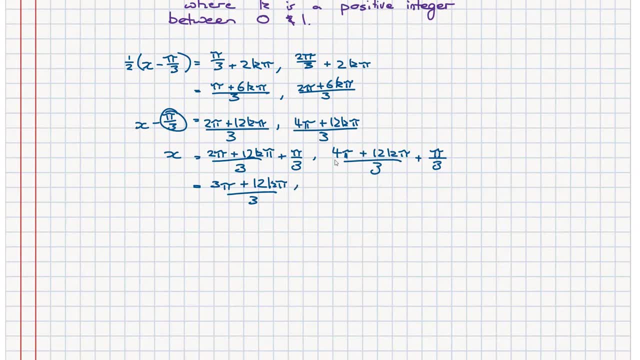 12k pi plus 12k pi all over 3, and then we're going to have 4 pi plus 12k pi all over 3, and then we can say not 4 pi, but 5 pi plus 12k pi all over 3, and then these are nice numbers here. so what I'll? 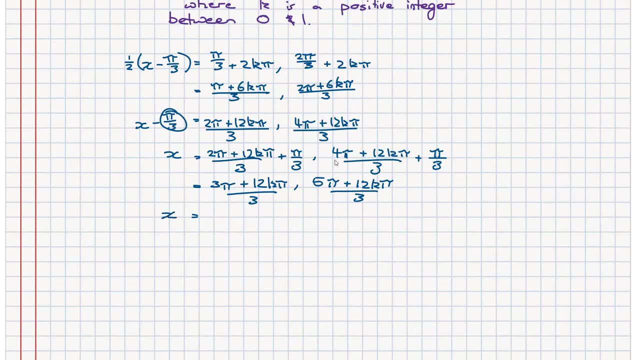 do is I'll get rid of the denominator and divide everything through, so it will be pi plus pi over 4k pi, and then- I can't do anything about this- 5 pi. so what I'll do is I'll just leave that as is for now, and remembering that k is equal to 0 all the way up to 1, so all the integers between 0 and. 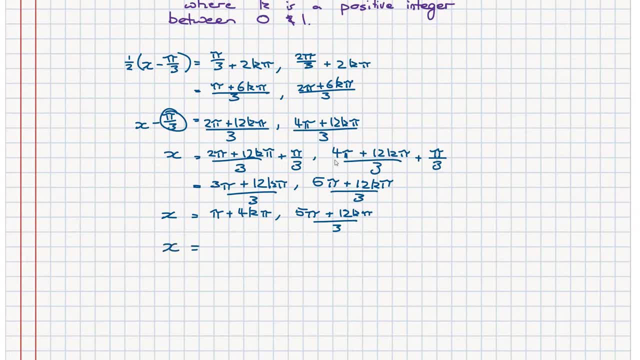 1. so we can say all of our solutions are going to be pi plus 4k pi. where k is 0, it's going to be simply 5 pi plus 12k pi all over 3, and then we're going to have 4 pi plus 12k pi all over 3 and